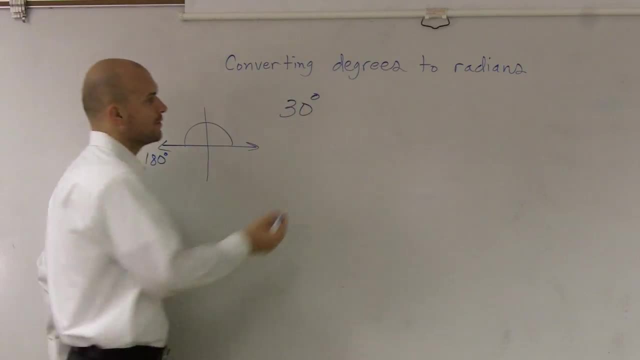 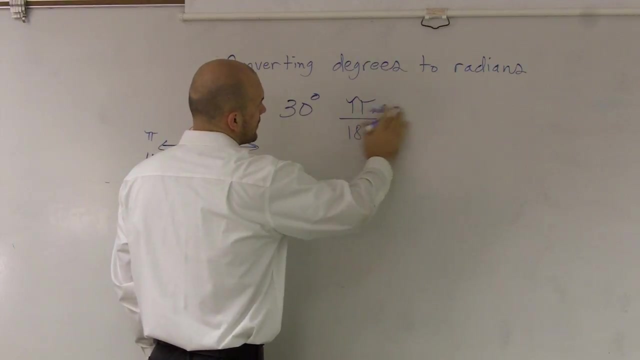 So when I want to convert from degrees to radians, what I'm going to do is I'm going to use that ratio. I'm going to say pi is to 180.. All right, And so this is what we call our pretty much our radian. All right, And here's what we're going to call our degrees. 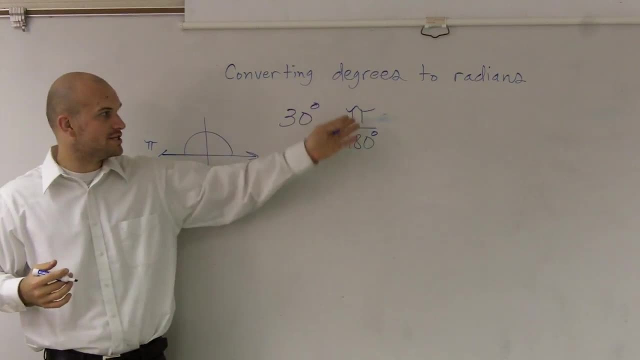 Oh, I get it. So now, the reason why I want to use this ratio as pi over 180 is because, remember, if I take a degree and I divide it by a degree, that's what's going to happen. is I'm going? 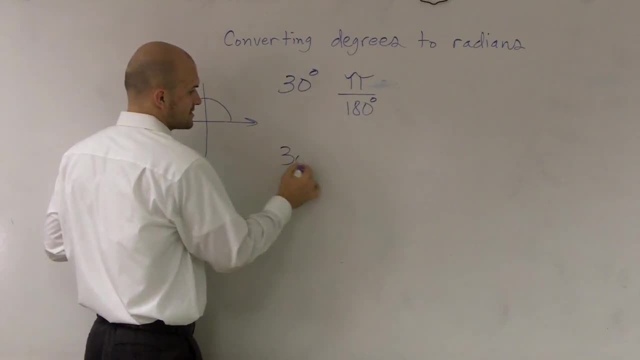 to cancel out And look at it this way. If you guys- for those of you that are physics people- let's say: this is radians, right, What pi radian is the same thing as 180 degrees, right, And I'll call this a degree as well. So, therefore, what happens is what a degree? 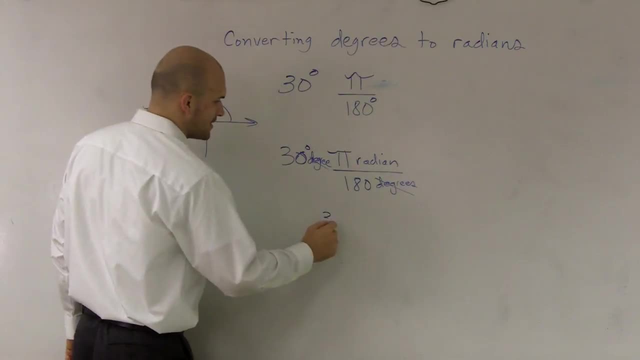 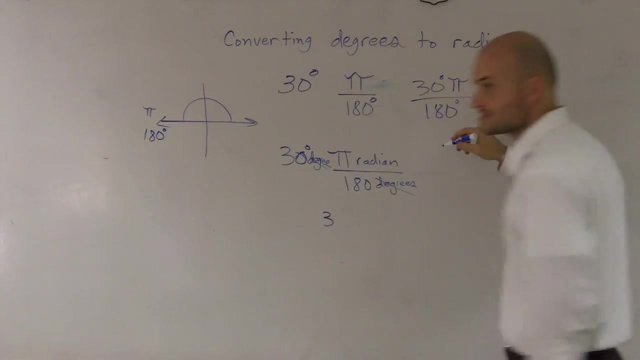 divided, a degree cancels out, right, And I'm left with 30 pi, 30 degrees pi over 180.. Well, this you can divide, you can simplify this fraction, right? The degrees actually cancel out, as I showed you. right, The degrees cancel out Physics, science, right, Chemistry you. 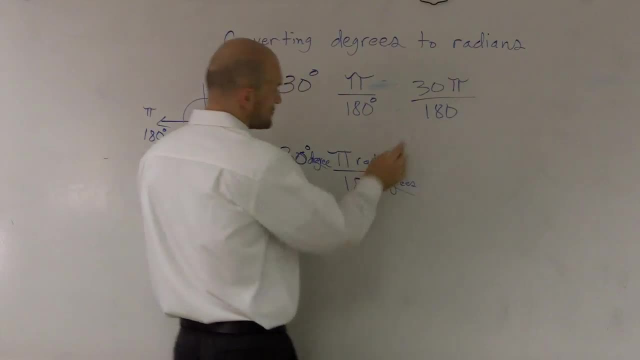 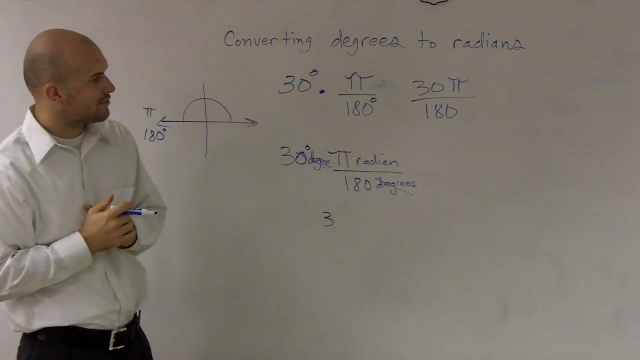 guys see that kind of stuff, Yes. So therefore, what we get is we're just left with our radian So 30 times pi, and then I can reduce this, So 30 goes into 180, what is that? Six times? 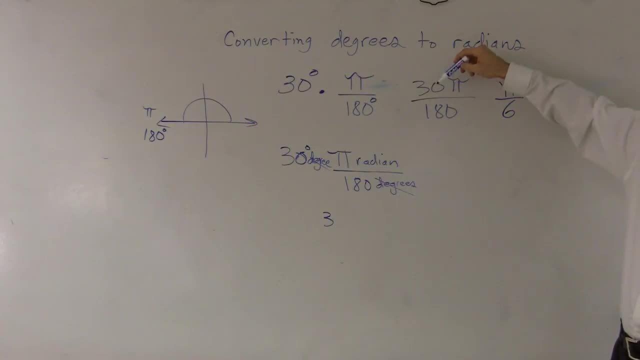 Well, think about it. What I'm doing is I'm dividing the top and bottom by 30,, actually not three. So, yes, it could be 10 over 60,, which reduces down to 1 over 6,, right So? 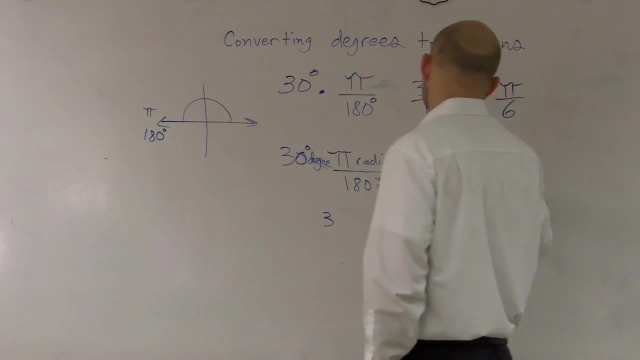 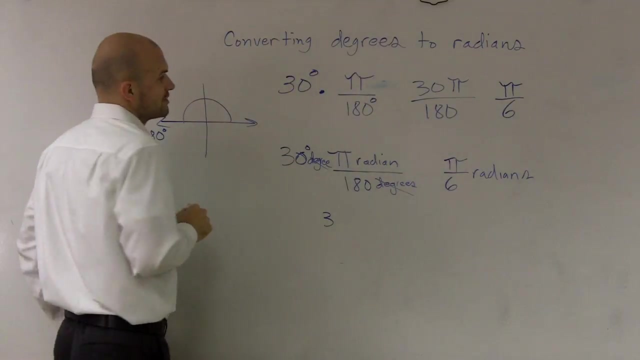 therefore it's pi over 6 radians. So therefore, what I have just done is- I have my answer, converting degrees to degrees radians. So what is 30 degrees? 30 degrees is the same thing as pi over 6 radians. We. 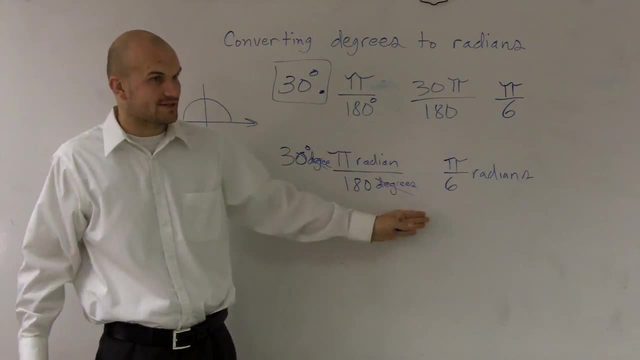 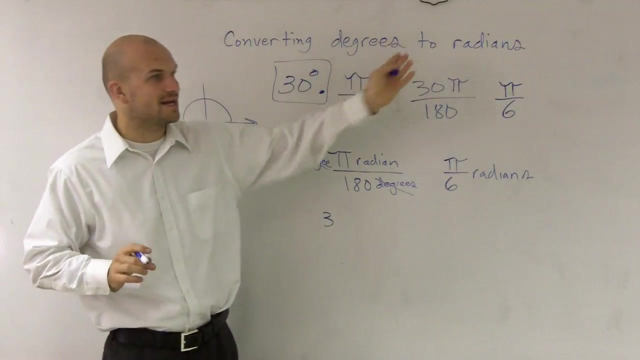 don't really write the radians part, but you guys now understand how the degrees cancel out to give us our radian. Does that kind of make sense? Yeah, So think of whatever you're doing when I say: convert to degrees, to radians, use the.